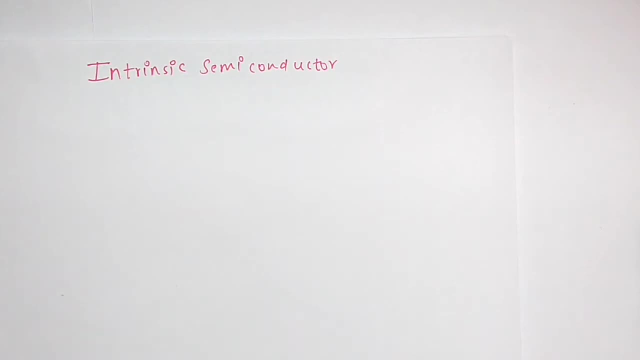 So in this video we are going to see what is done by intrinsic semiconductor and extrinsic semiconductor, As we discussed earlier. the pure form of semiconductor is called intrinsic semiconductor. For example, it is silicon and germanium. Let's take a silicon atom. 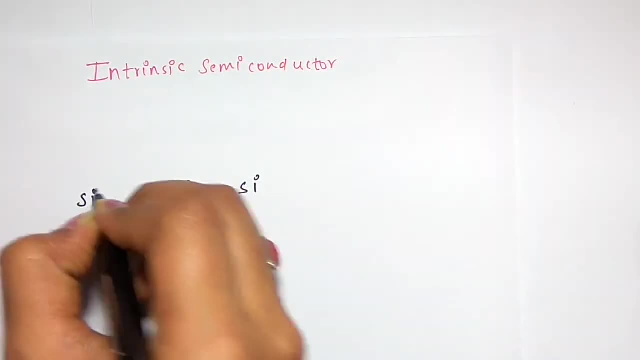 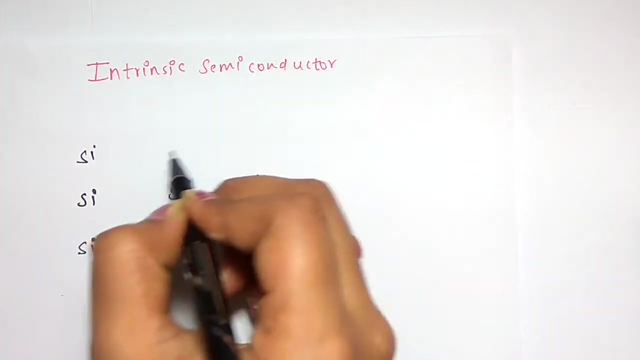 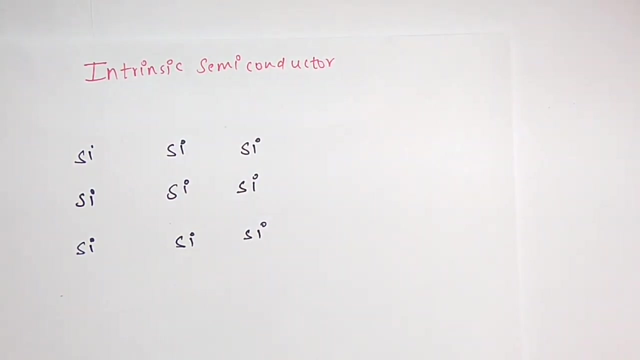 So generally, the valency of silicon is 4.. As it is the fourth group element, the valency will be 4.. So this is the valency electron. So we know that the four valency electrons of silicon forms four covalent bonds with the nearest four silicon atoms. 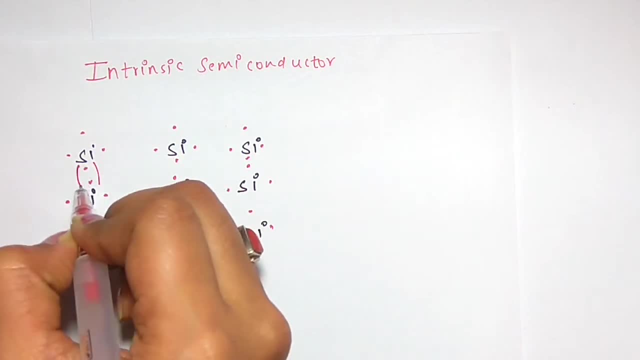 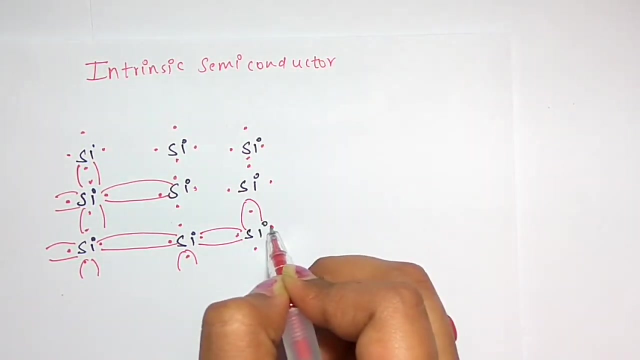 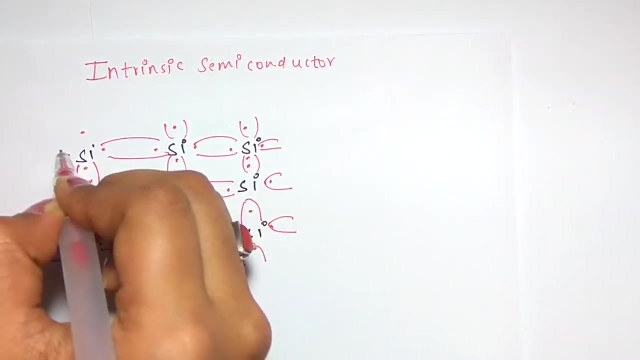 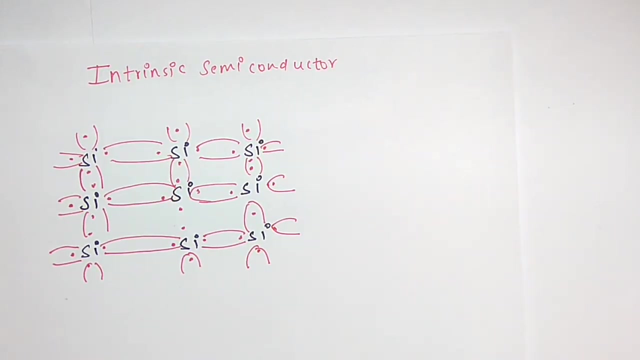 So this is the covalent bond. It shares and forms the covalent bond with the nearest silicon atom, So every electron is in bonding. now No electron is free here, So every electron participates in bonding. So the four valency electrons of silicon forms four covalent bonds with the nearest four Webb signals. 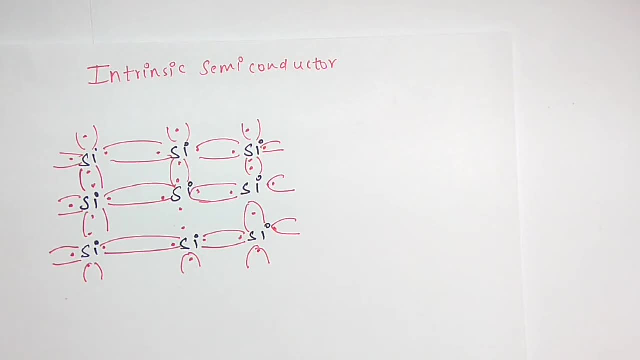 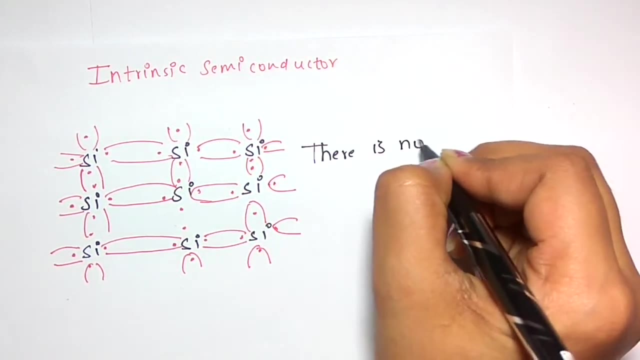 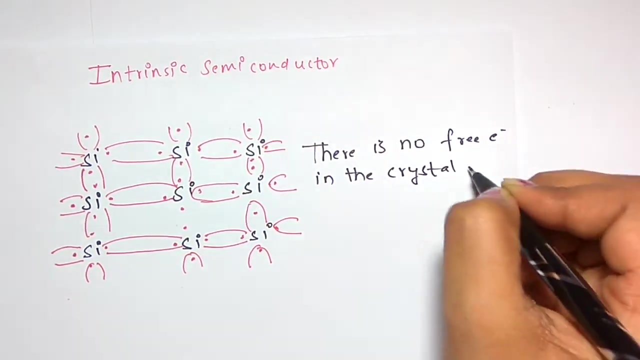 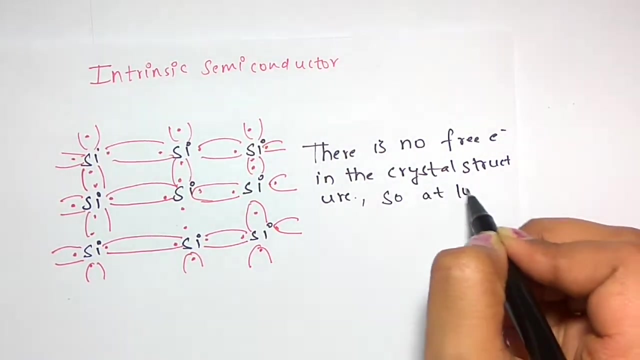 So this is the covalent bond with the nearest four silicon atoms. There is no free electron in the crystal structure. So there is no free electron in the crystal structure. So at low temperature, that is, at 0 Kelvin, the semiconductor behaves like insulator. The semiconductor because, as there is no free electrons there, 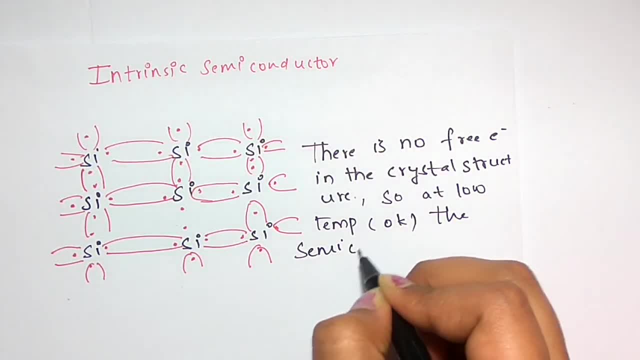 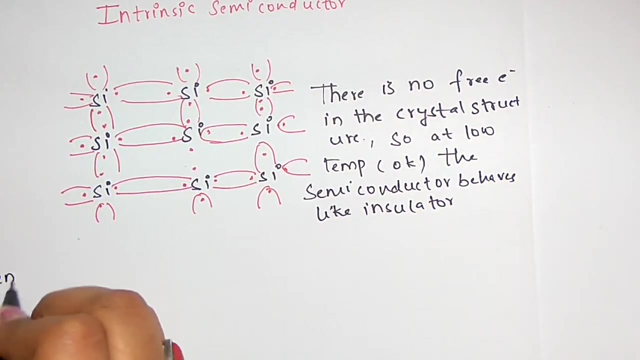 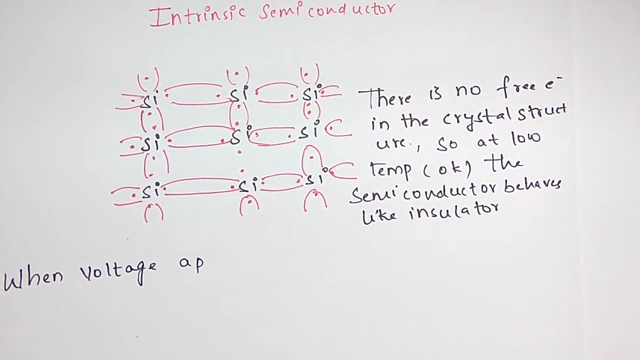 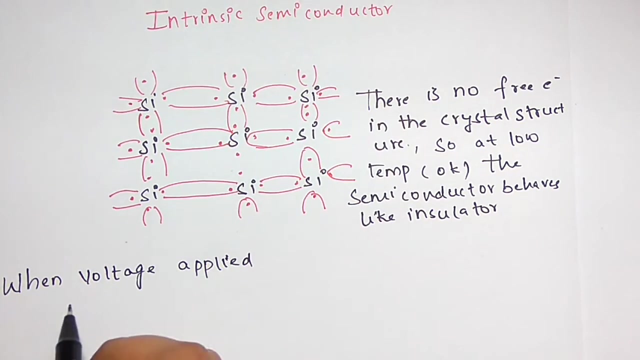 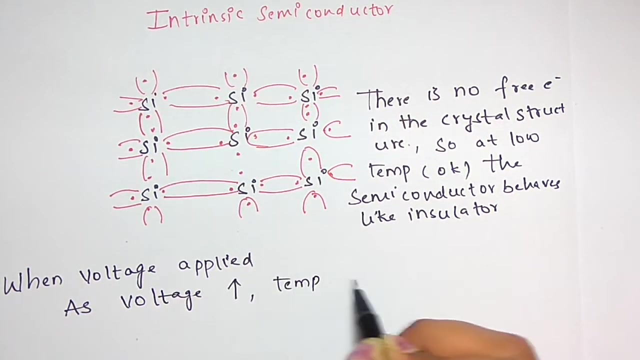 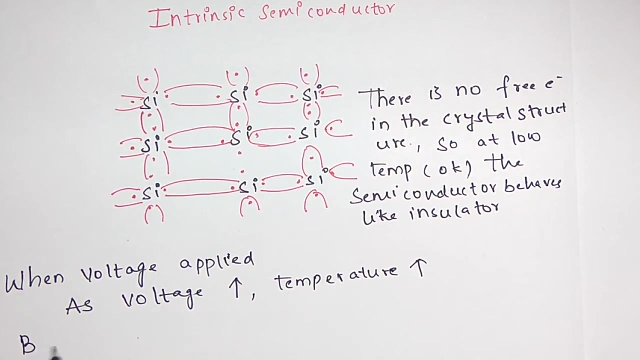 is no flow of electrons, that means there is no electrons. The semiconductor behaves like insulator, Suppose when we apply voltage, When voltage applied, When voltage applied, So as voltage increases. So here we are applying voltage So as voltage increases, temperature increases. Temperature increases, Breakage of covalent bond increases As the temperature. 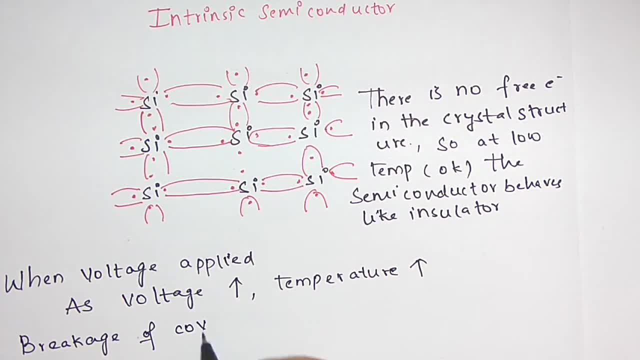 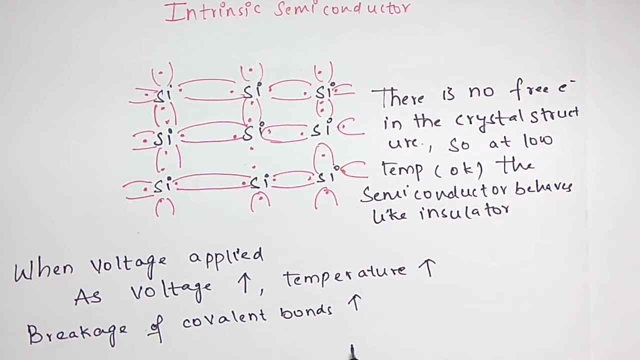 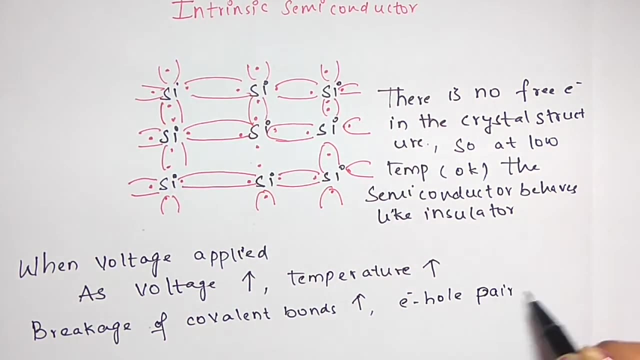 increases breakage of covalent bond increases. If breakage of covalent bond increases, what will happen? Electron hole pair will generate Electron hole pair generation increases. So what happens if electron hole pair generation increases? that means there are more number of free electrons. So if free electrons are, 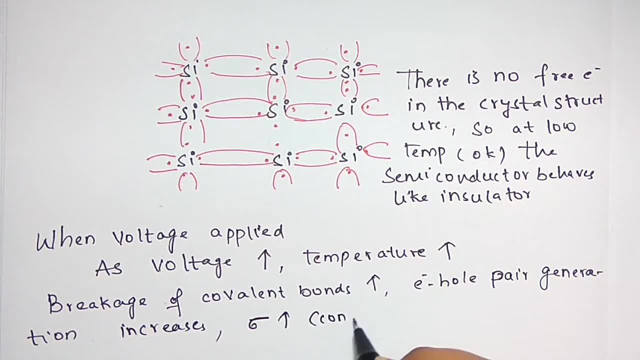 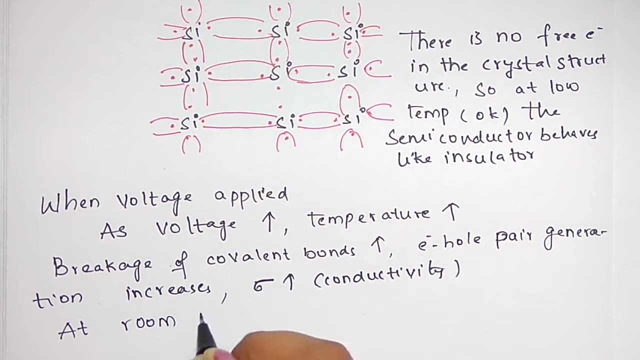 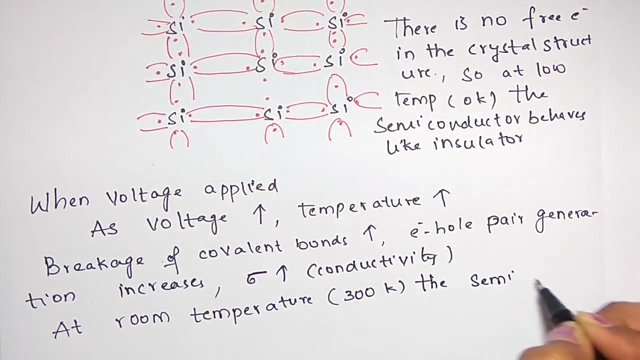 there conductivity increases. Sigma means conductivity Conductivity increases. So this is the condition. So at room temperature that means, as voltage increases, temperature increases. Suppose it reaches to room temperature. At room temperature, say 300 Kelvin, the semiconductor behaves like now. conductor: The semiconductor behaves like now. So this is the condition. So at room. 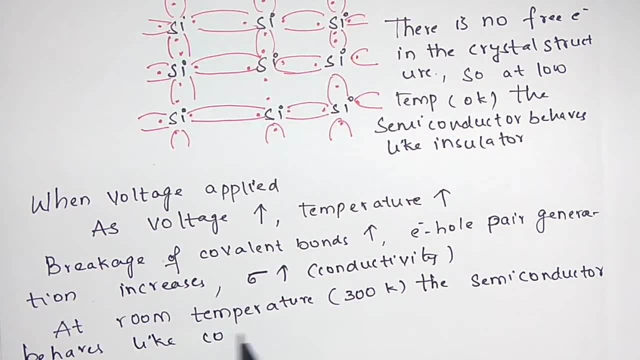 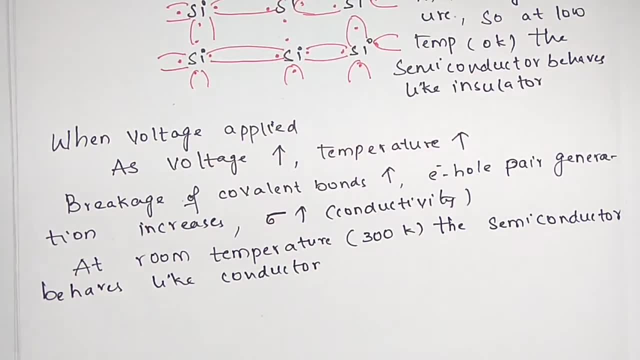 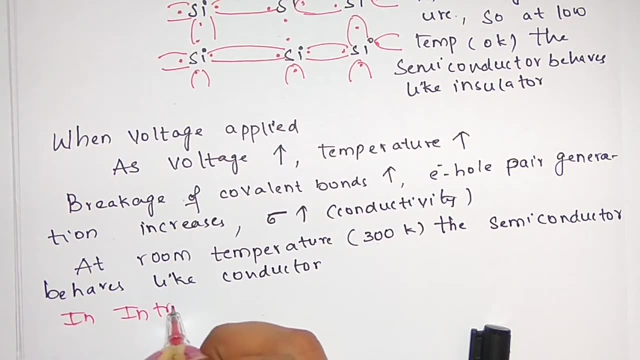 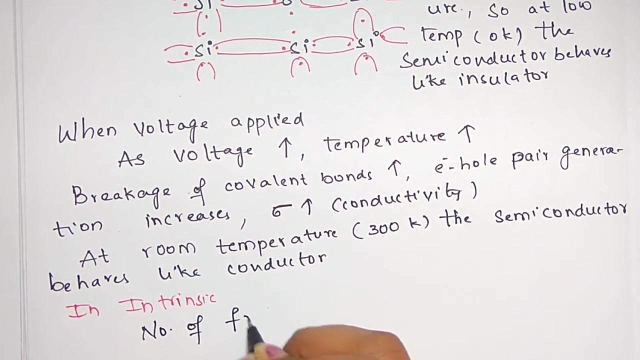 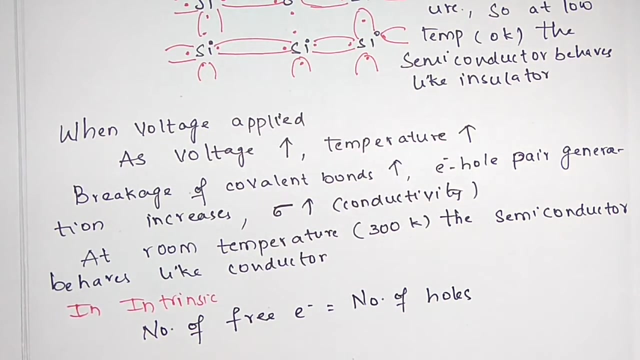 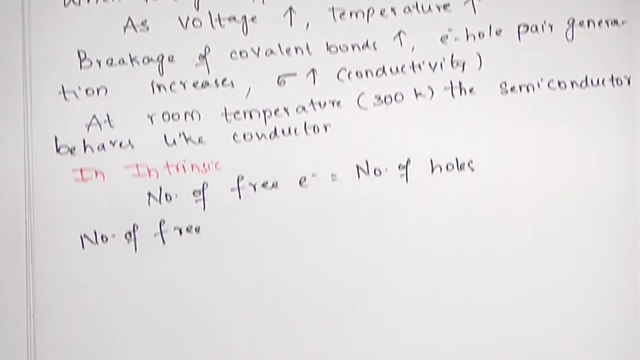 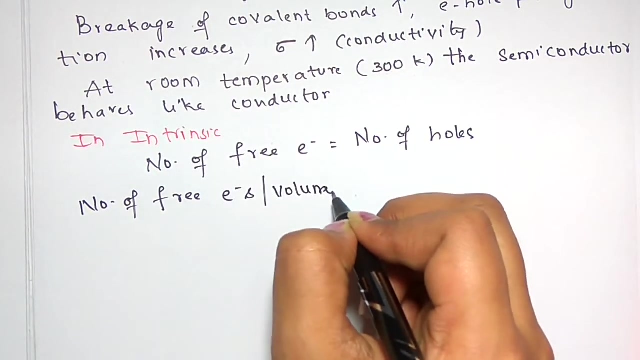 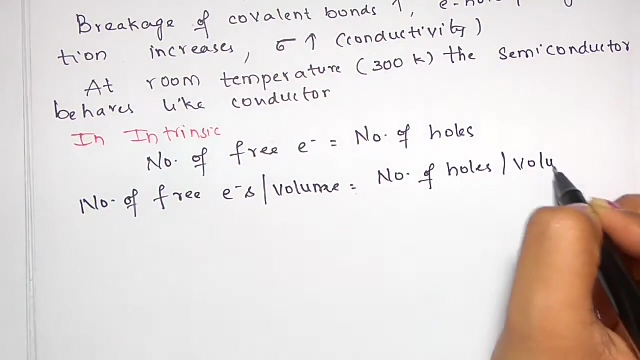 behaves like conductor. So this is about intrinsic semiconductor. So generally, in intrinsic, number of free electrons is equals to number of holes. So you can also say that number of free electrons- free electrons per volume, is equals to number of holes per volume. So nothing but number of free electrons per volume is. we can say: 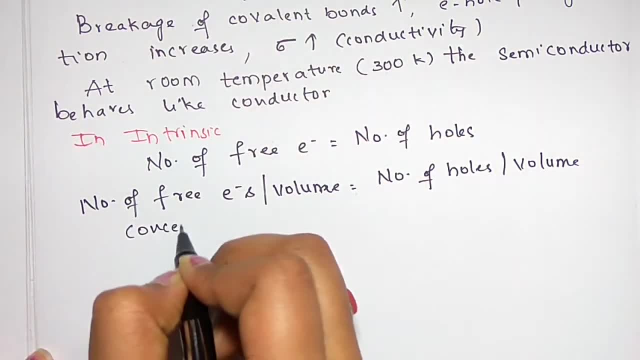 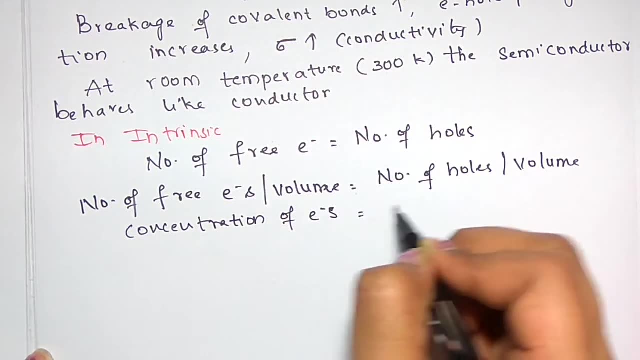 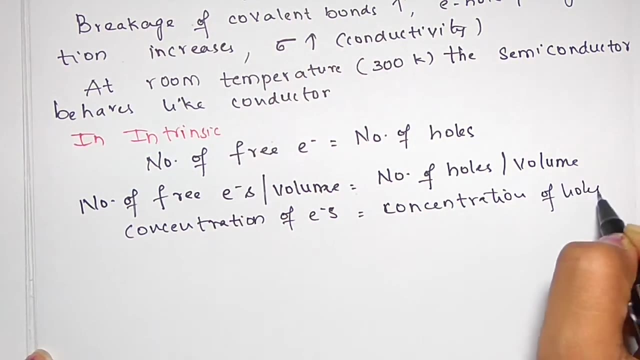 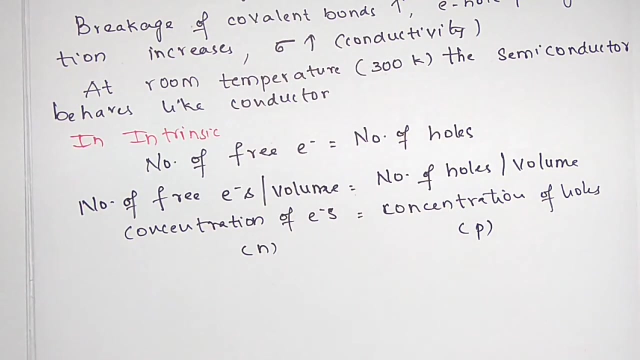 it as concentration of electrons. So concentration of electrons, So concentration of electrons, is equals to concentration of holes. So in intrinsic type, concentration of electrons, say n, concentration of holes, say p. So n is equals to p. So according to mass action law, mass action law. 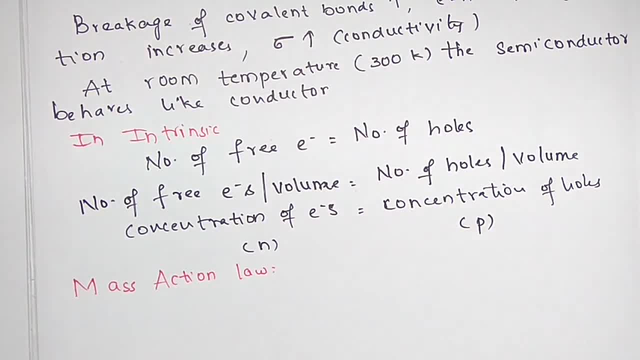 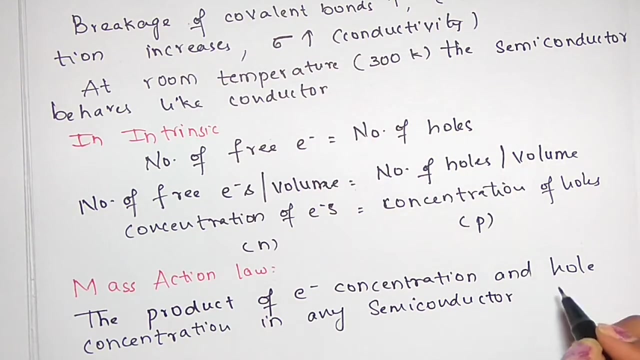 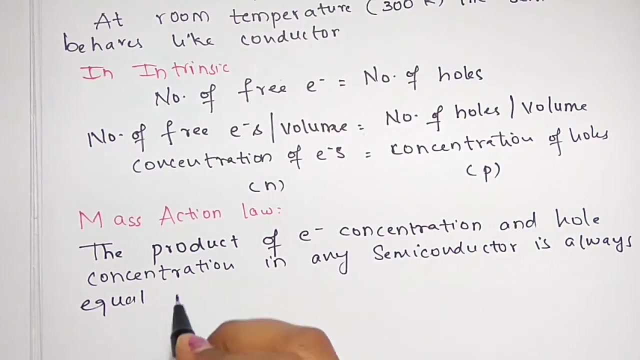 the product of electron concentration and hole concentration in any semiconductor is always equal to square of the intrinsic semiconductor concentration. So I will repeat again: The product of electron concentration and hole concentration, concentration in any semiconductor, in any semiconductor, is always equal to, is always equal to square of the intrinsic semiconductor concentration, intrinsic. 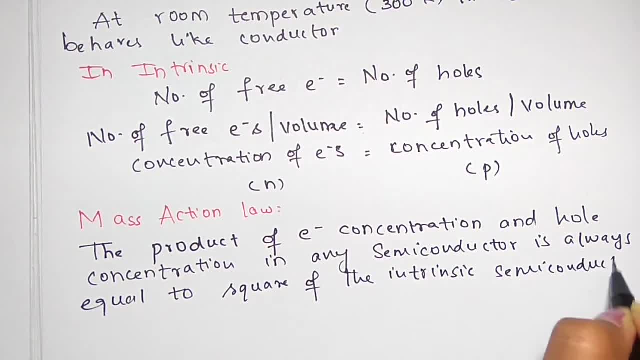 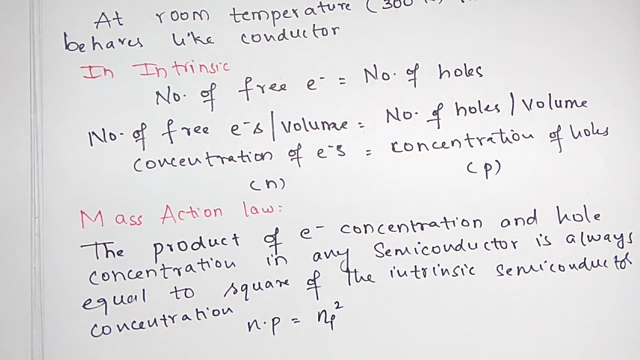 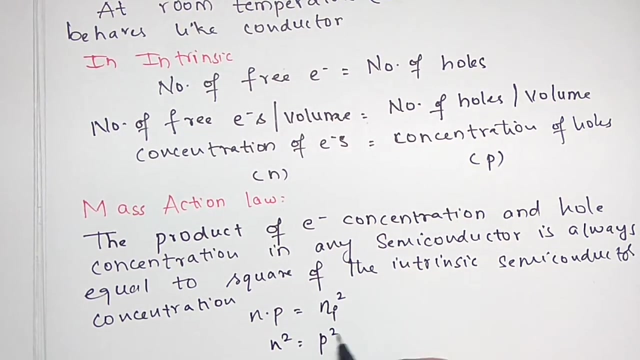 semiconductor concentration. so see, electron concentration is n whole concentration is p product of n into p equals to intrinsic semiconductor concentration square. so suppose it is ni, ni square. so you can also write it as we know that in intrinsic semiconductor n is equal to p, so n square equals to p square equal to: 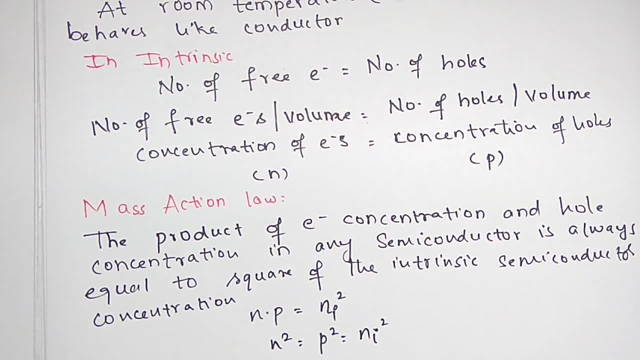 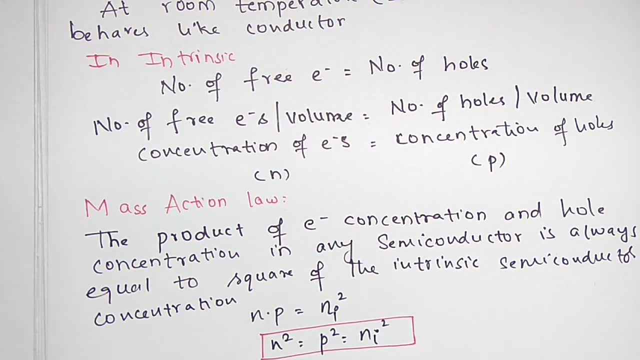 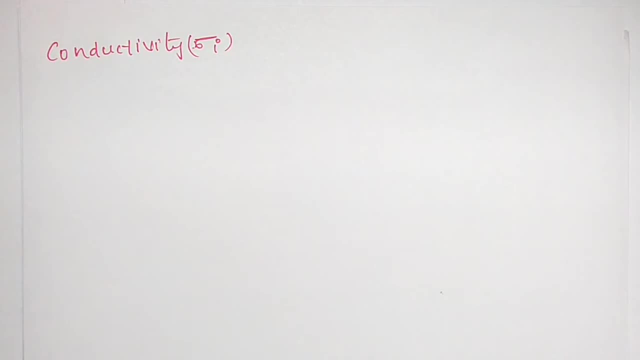 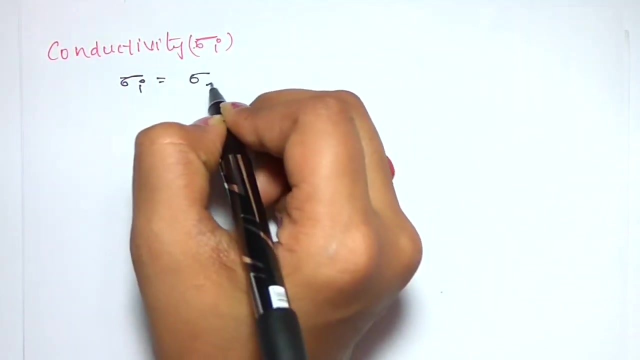 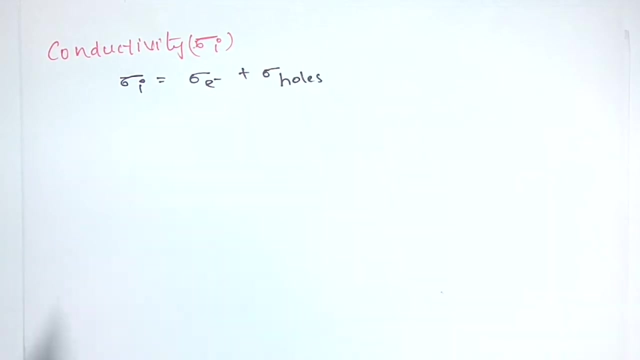 ni square. so this is next coming to conductivity. conductivity of intrinsic semiconductor, sigma i, is equals to nothing but conductivity contributed by electrons plus conductivity by holes. so generally conductivity formula can witness number of electrons, concentration into charge of electron, into mobility of electron, similarly concentration of holes into charge of. 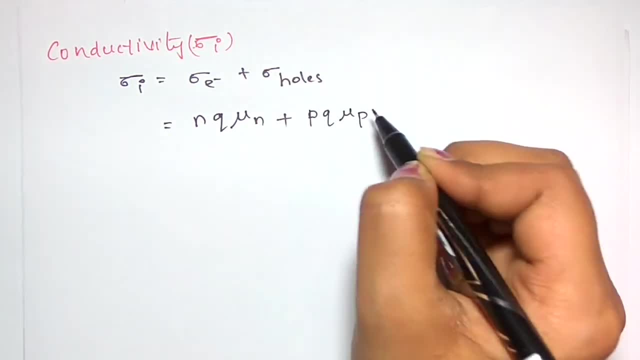 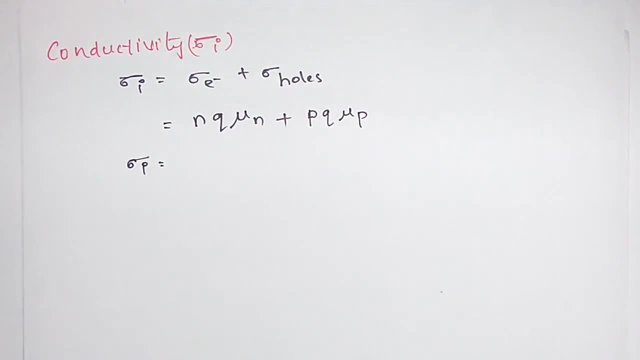 holes into mobility of holes. this is the conductivity formula, but we know that in intrinsic semiconductor then n equals to p is equals to ni, so you can write it as ni cube mu n plus mu b mu p, mu p, mu p mu v, mu p mu i. 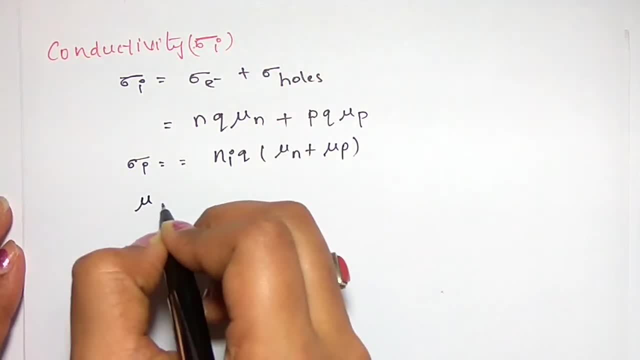 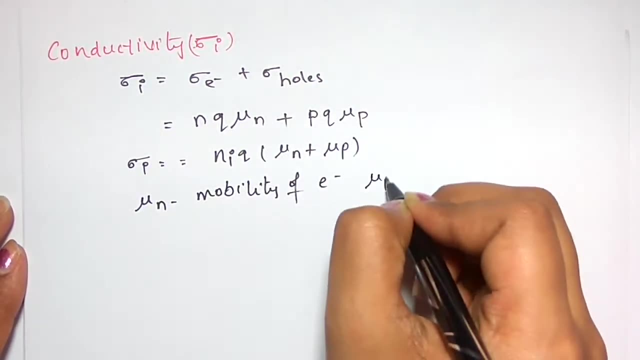 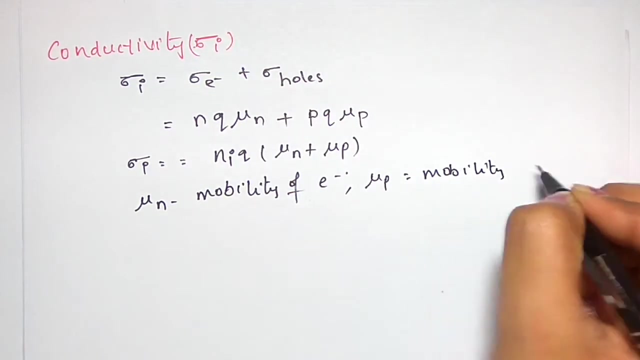 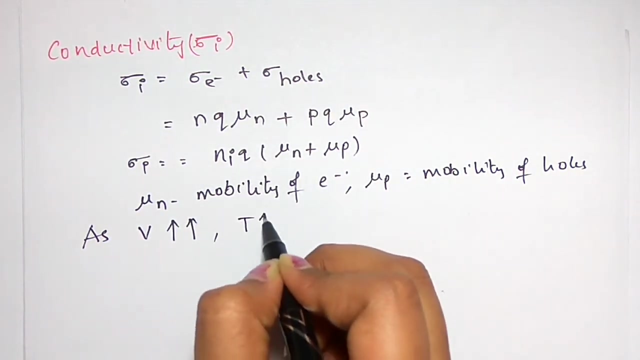 mu n, mu a, mu b and mu p are. mu means mobility of electron, mobility of electron, mu, p means mobility of holes. So we know that as voltage increases- suppose if we further increase voltage, as voltage increases, temperature further increases, breakage of covalent bond further increases- 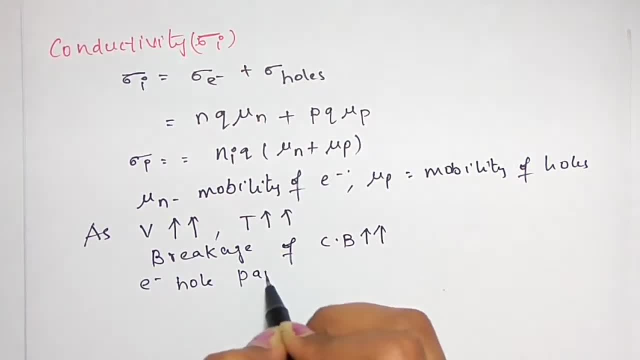 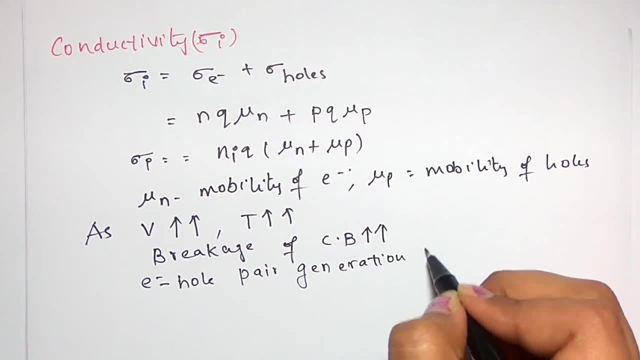 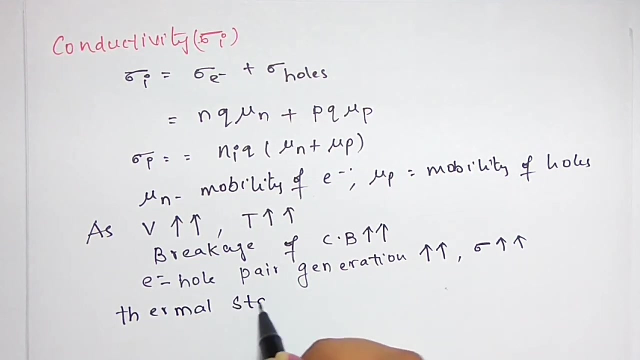 electron hole pair generation increases if electron hole pair generation increases conductivity. If temperature is increased more, then thermal stability will be less, So the stability of the element will be decreased. if the temperature is more And at some particular voltage, the generated temperature becomes large, 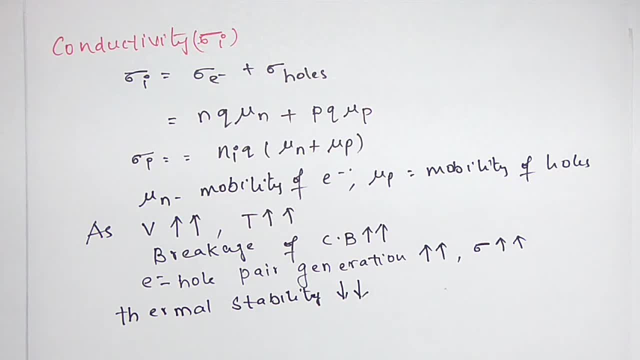 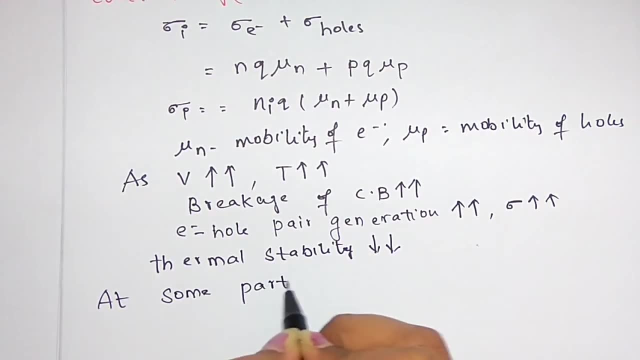 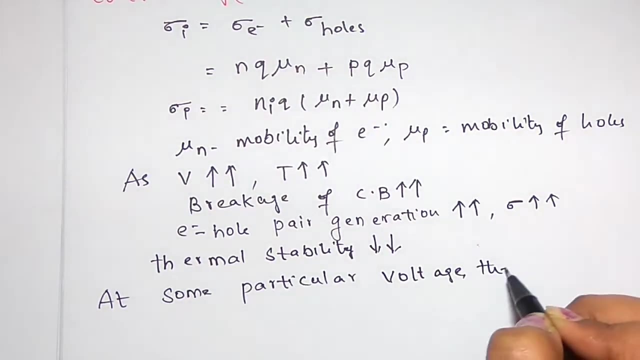 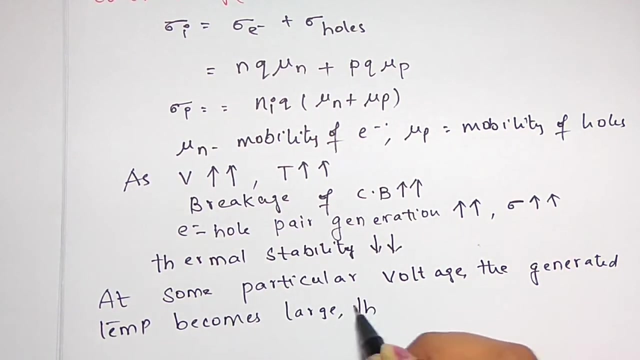 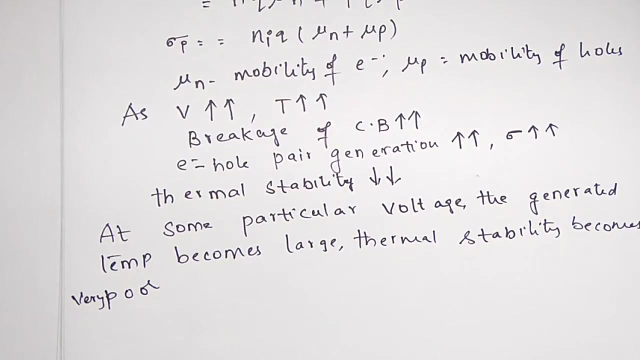 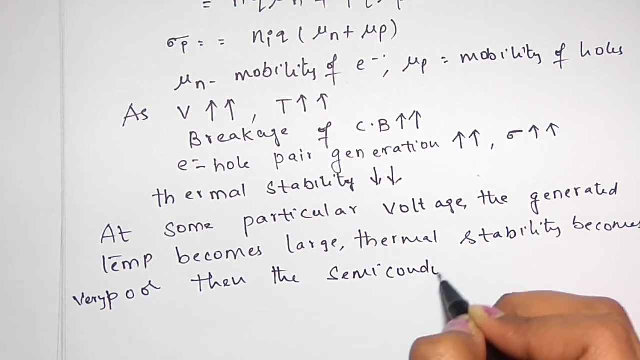 Thermal stability becomes very poor, Then the semiconductor permanently damages. At some particular voltage the generated temperature becomes large. Thermal stability becomes very poor. Thermal stability, Thermal stability becomes very poor, Then the semiconductor permanently damages. Then the semiconductor permanently damages, So without applying much external energy. 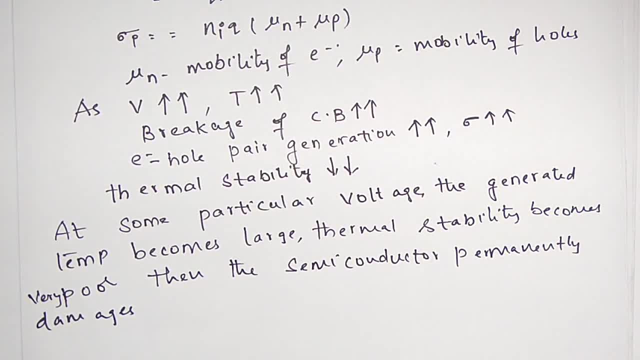 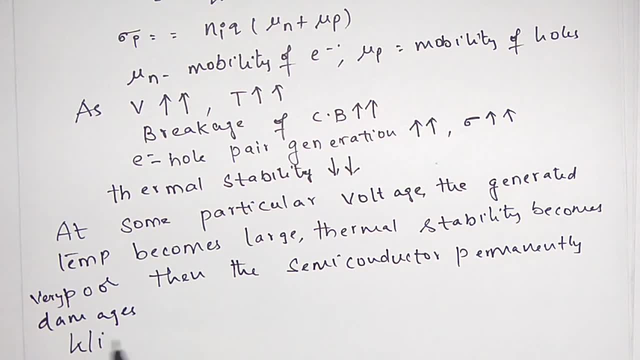 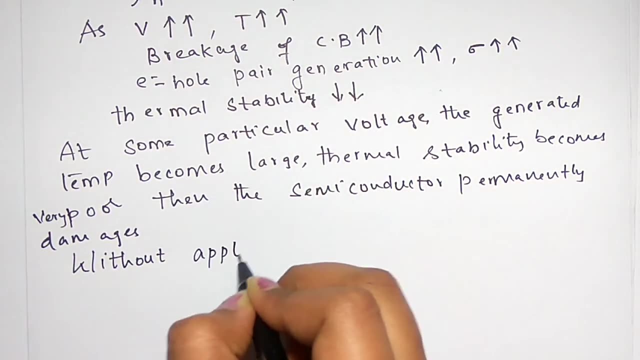 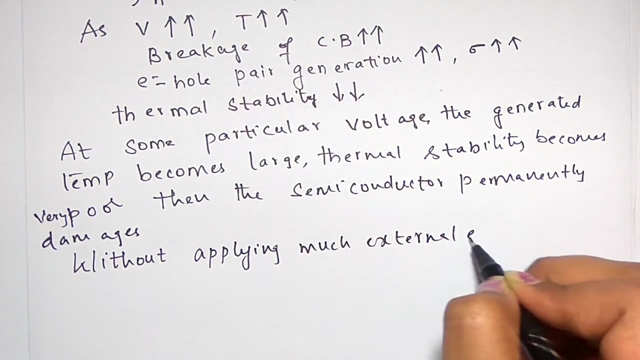 So in intrinsic semiconductor, if you apply external energy only, then only it will conduct. But if you apply more energy, what will happen? The semiconductor permanently damages. That's why, without applying much energy, much external energy, to get more conductivity, 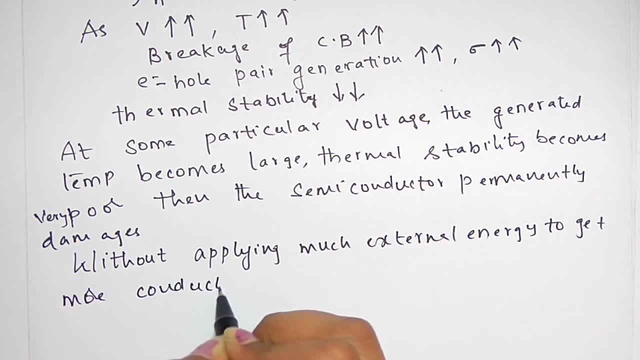 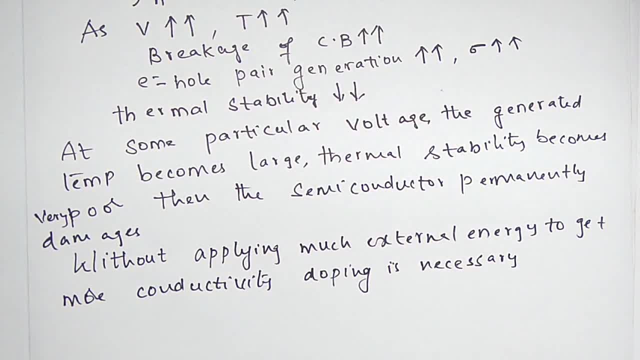 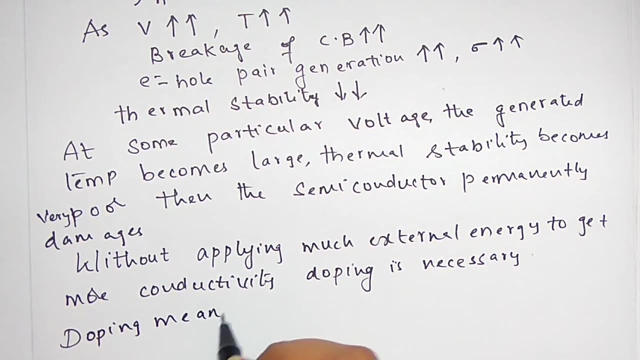 So the semiconductor loses its thermal stability and it will be damaged. That's why, without applying external energy, but still if we want to increase conductivity, doping is necessary. So what is meant by doping? Doping means addition of impurities.